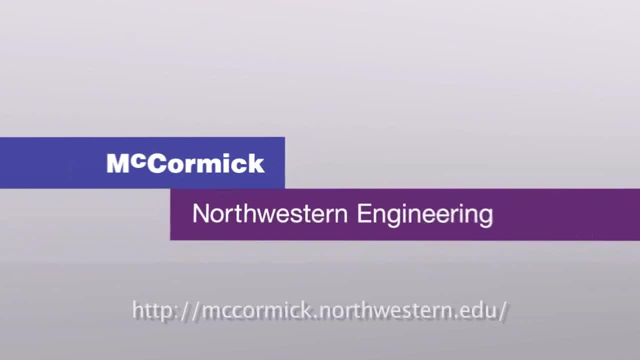 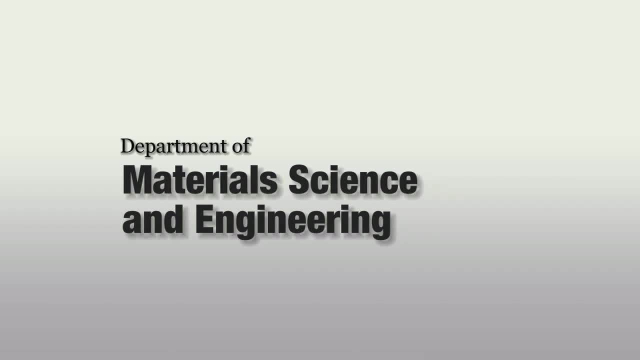 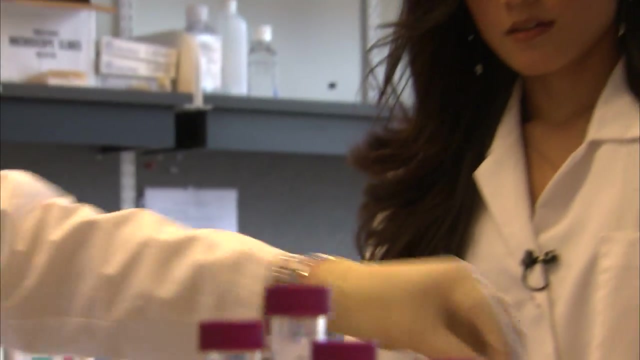 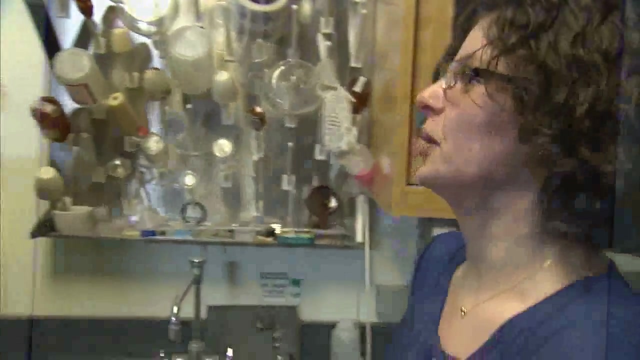 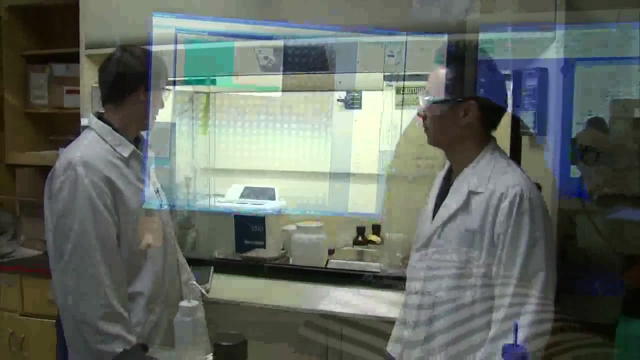 Established over 50 years ago as the first material science department in the world, the Department of Material Science and Engineering at Northwestern University's McCormick School of Engineering continues to lead the field and is ranked among the top programs in the country. The field is dynamic because understanding materials is the basis for all technology. 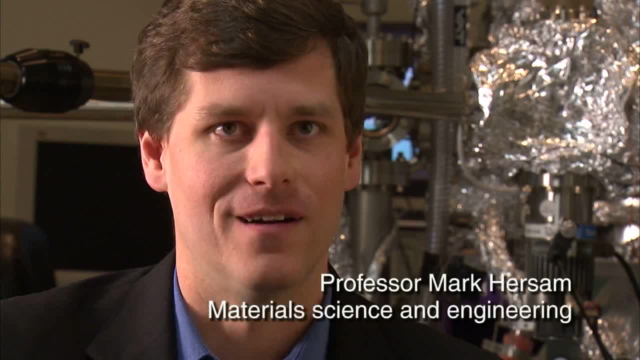 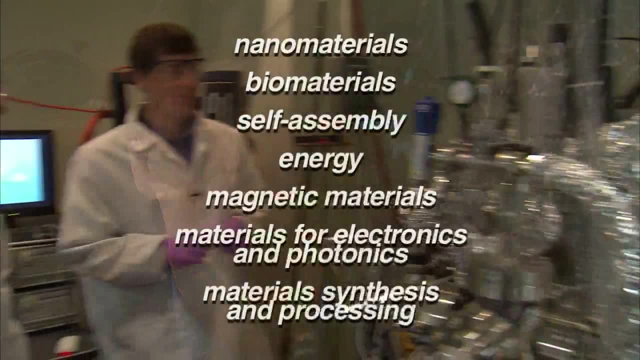 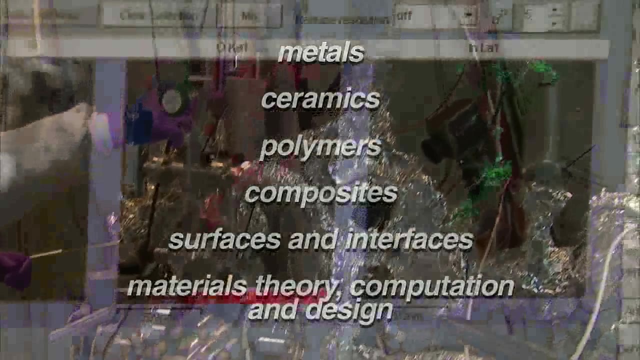 The fundamental premise of material science is that the structure of matter leads to its properties. So if we can control structure at the atomic scale, then we should be able to engineer whatever property we want. Faculty members have been honored worldwide for their pioneering research, which spans the entire spectrum of materials research. This video 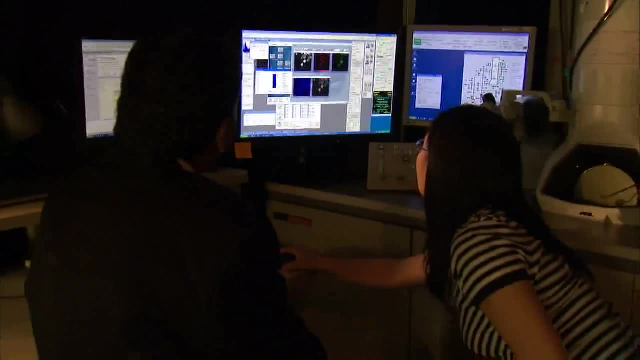 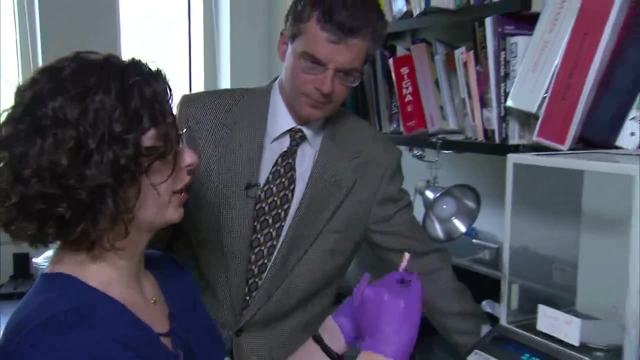 will highlight only a few of the department's faculty and current research projects. David Dunant is an expert in metals. He is working on the development of strong, lightweight, energy-absorbing metal foams. We're now making aluminum foams. This is an 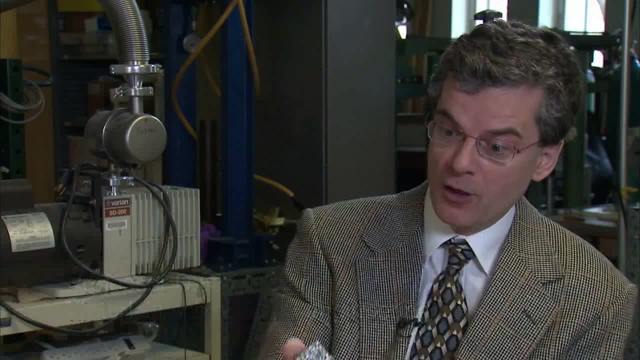 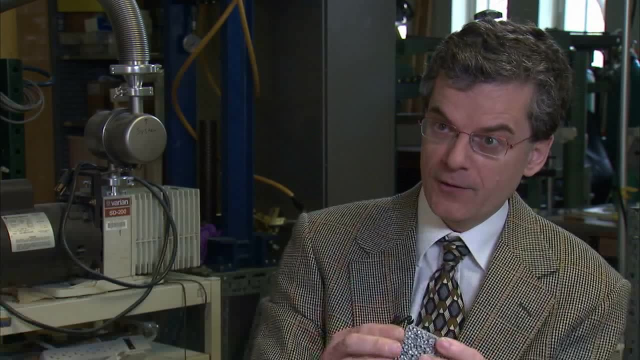 example of an aluminum foam. It's extremely light. It would certainly float on water in that particular case- And just like a styrofoam- now, if you squish it it absorbs a lot of energy. So you can think of using this, for instance, for very lightweight bumpers for cars. 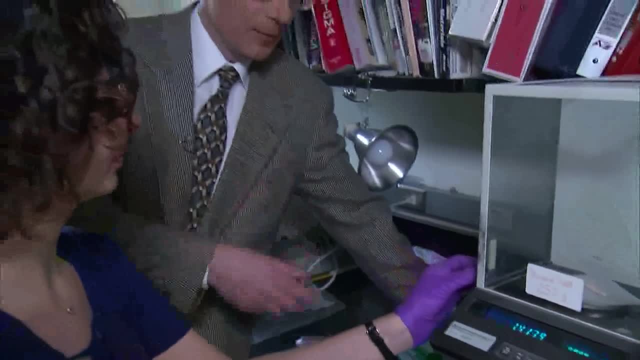 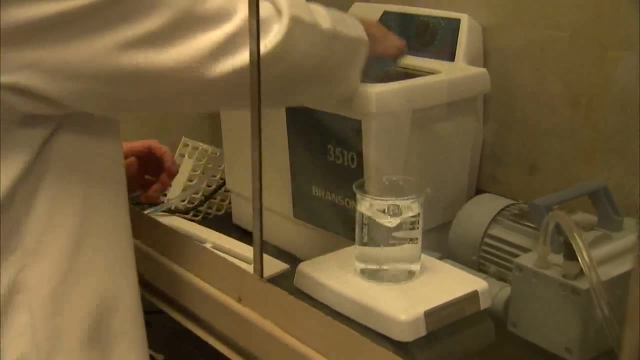 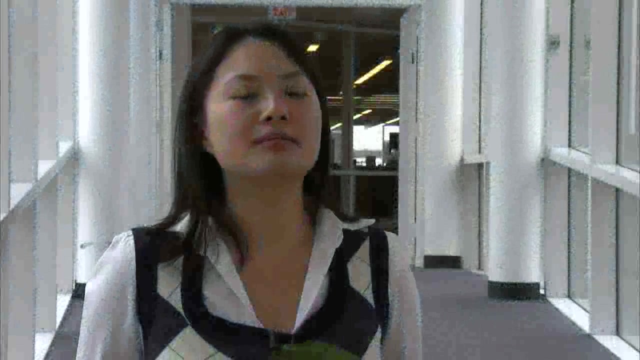 The combination of strength, lightness and absorption power could soon result in cars that are safer and more energy-efficient. Other faculty student research teams in the department are developing materials for use by the Navy. We're using fundamental data on titanium alloys to develop new high-strength. 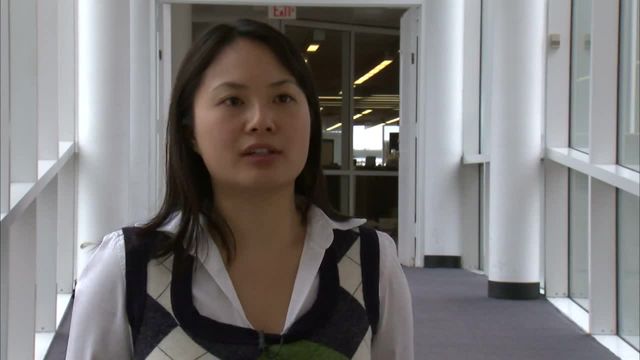 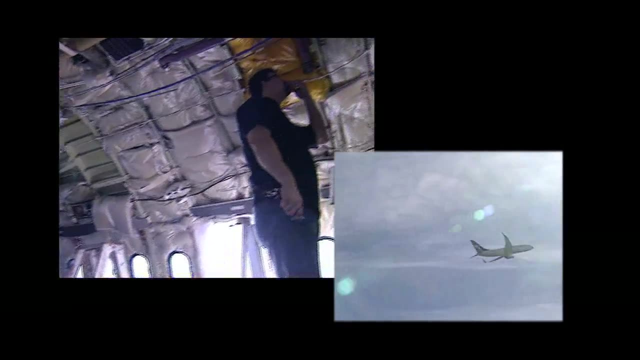 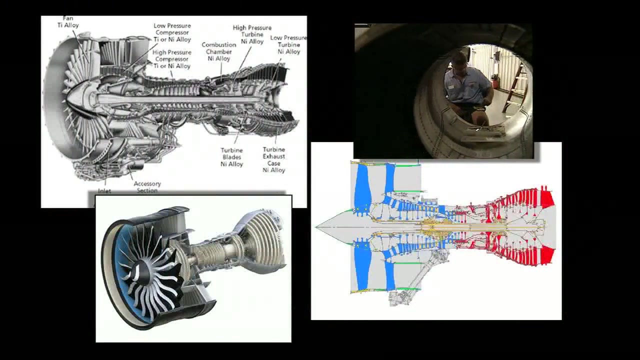 high-toughness alloys for applications such as lightweight, high-speed watercraft. Still other research teams are striving to develop more energy-efficient aircraft. I'm working on the nickel-based superalloys, which is the improvised alloys for the turbine engines. The goal is higher heat treatment temperatures and lower operating costs. 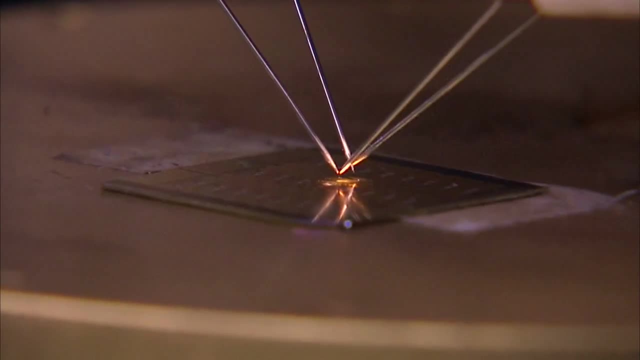 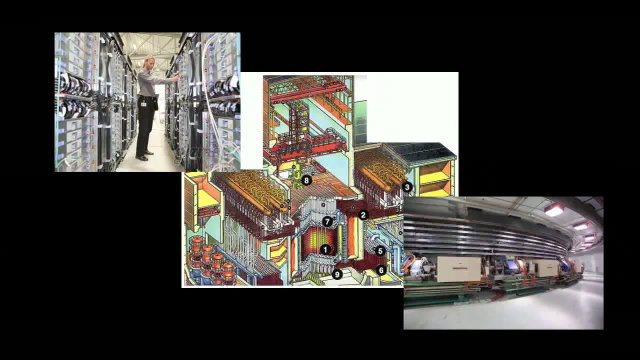 In its groundbreaking research, the department collaborates with national laboratories, especially nearby Argonne National Laboratory, where faculty member Mike Bedzik heads the Synchrotron Center at the Advanced Photon Source, one of the most powerful synchrotrons in the world. 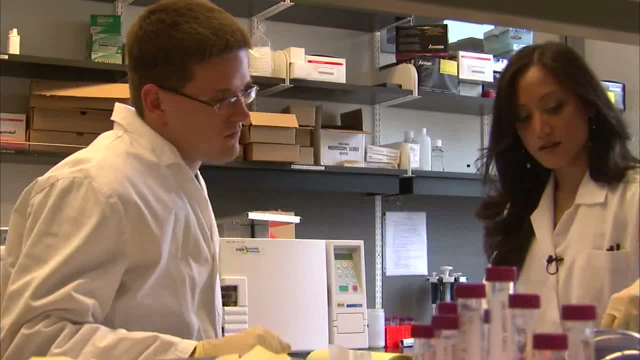 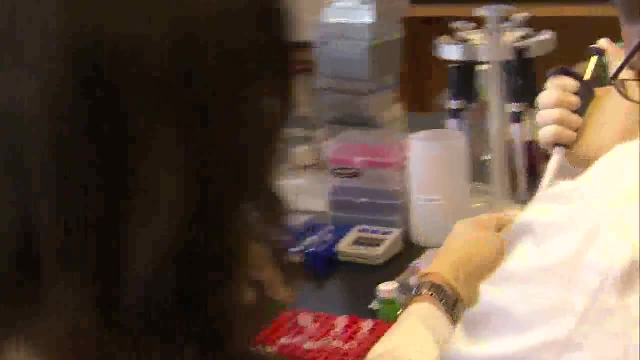 So we're going to do one that is a 3300.. Okay, Okay, And then the rest will be the 2000 molecular weight. yeah, Ramil Shah's research spans the emerging areas of nanomaterials, self-assembly and biomaterials. 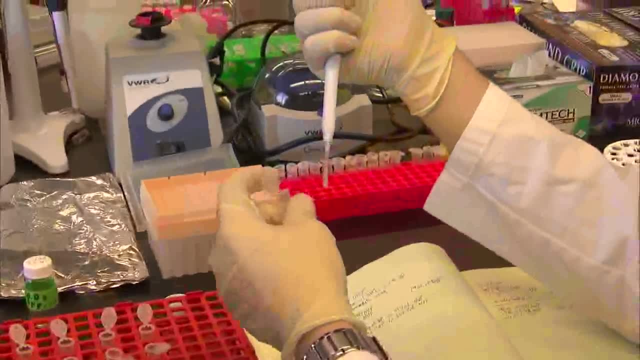 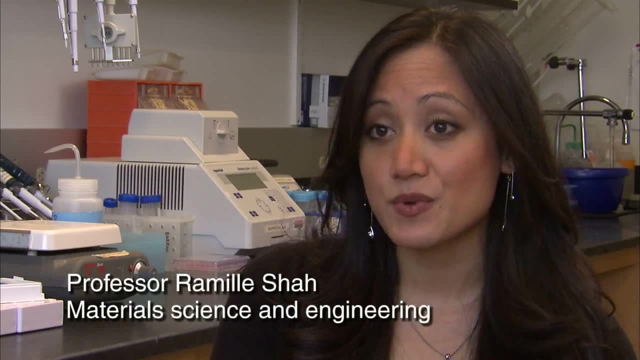 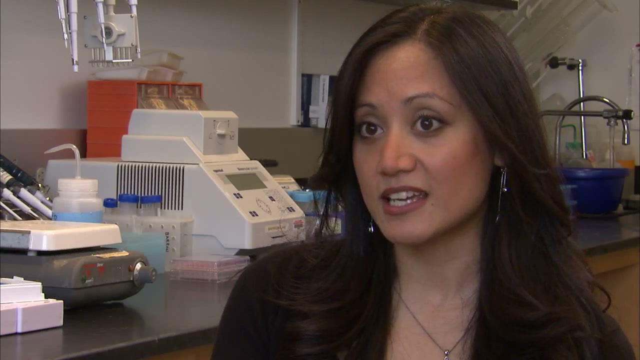 Her group focuses on developing novel biomaterials for use in regenerating damaged tissue or bone, Trying to create therapies, whether it be through injecting cells, whether it be through injecting or implanting materials, but really developing therapies that can be used in the 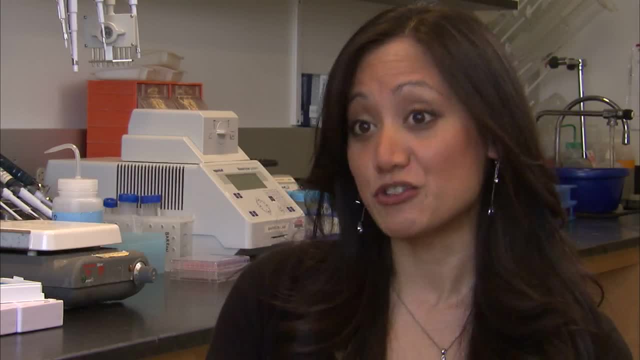 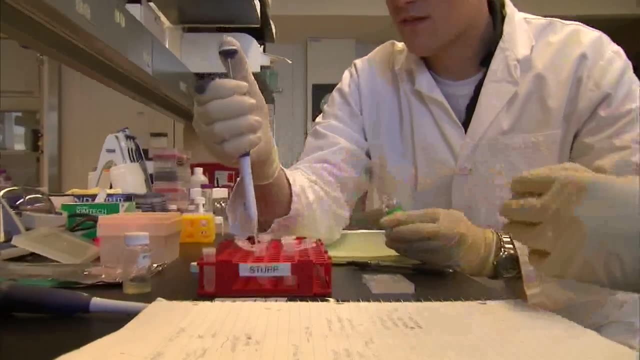 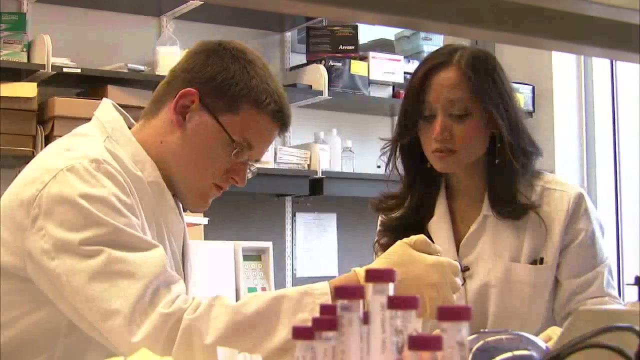 body, to sort of jump start the regenerative process in your own body. The aim is to reduce the need for invasive surgery, eliminate the need for placing metal parts in the body, alleviate suffering and promote quicker healing. The end goal is to really make an impact on patient quality of life. Doing this type of 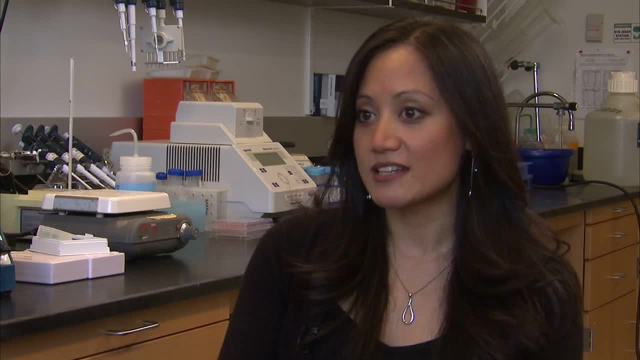 research developing materials for a clinical application is very motivating. We would proceed to vent the load lock via this nitrogen line. A lot of people have been saying that this is a very long-term thing. We're looking at it as a very long-term thing. We're looking at it as a long-term thing. We're looking 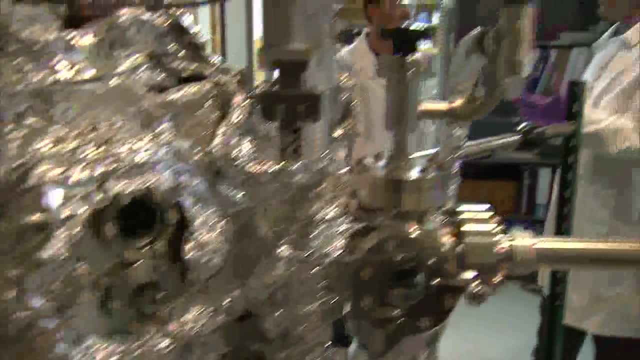 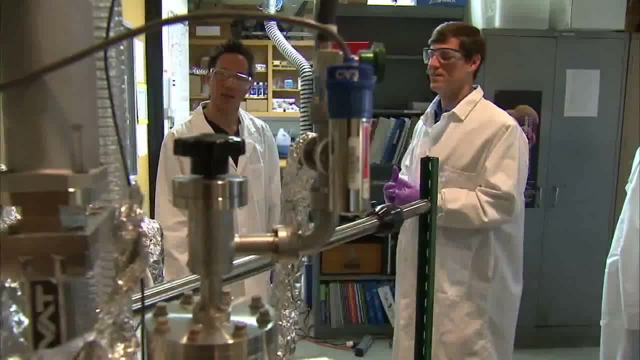 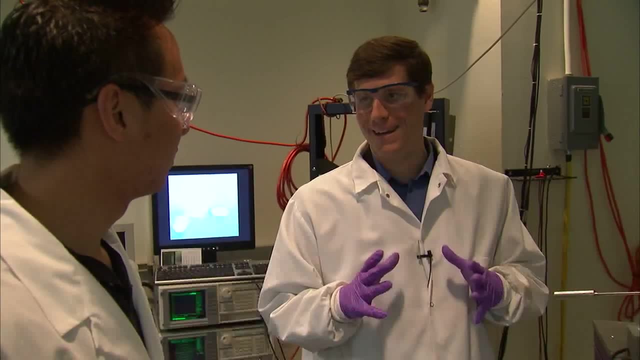 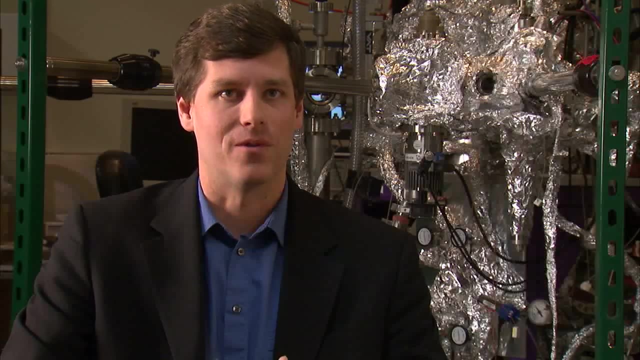 power of integrated computer circuits by reducing electronics to the atomic scale. Hersom and his research team have developed individual electronic devices that are a single nanometer in size. If you change the diameter of a carbon nanotube at the atomic scale, you can change its properties dramatically …. 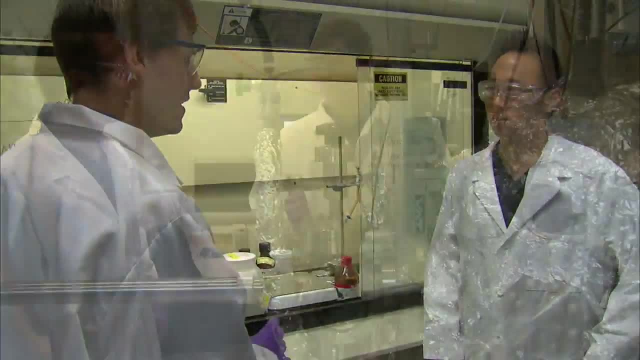 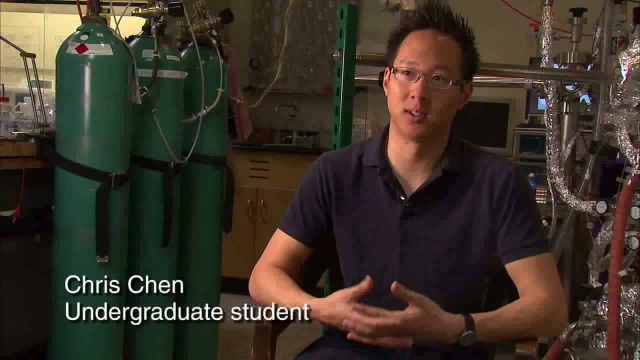 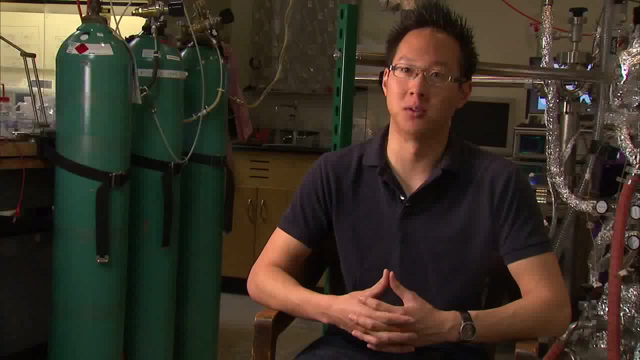 One of Hersom's undergraduate students, Chris Chen, is helping to develop transparent electronic controls on the nanometer scale. I've been working primarily on a class of materials known as transparent conducting oxides to pattern conductive wires, thus making transparent interconnects that could be used. 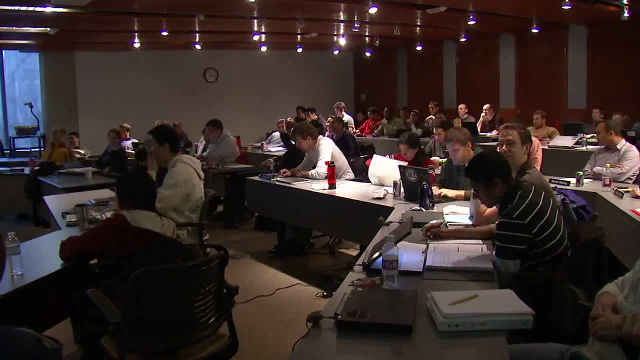 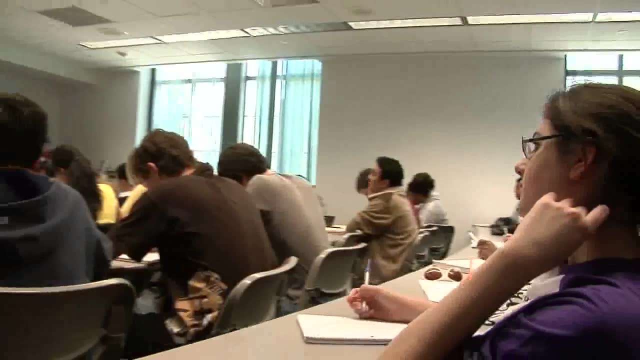 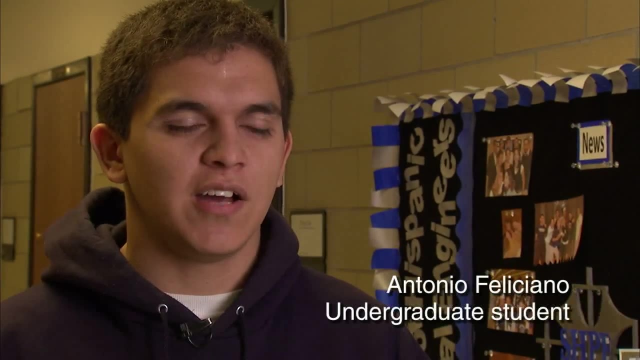 in electronics of the future. The undergraduate program gives students the fundamental tools to apply mathematics and science to a wide array of materials engineering problems. They also have the opportunity to become part of exciting research teams. The project I'm working on is actually for making sure that when you put a stent inside.